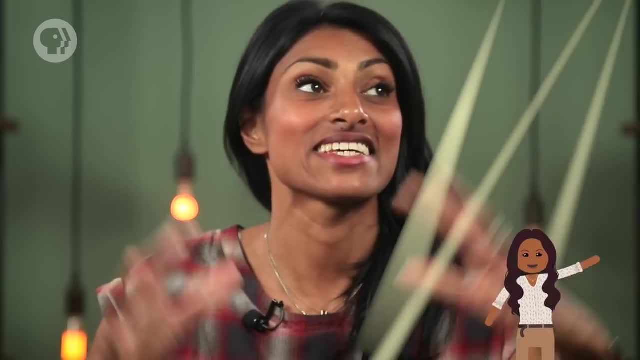 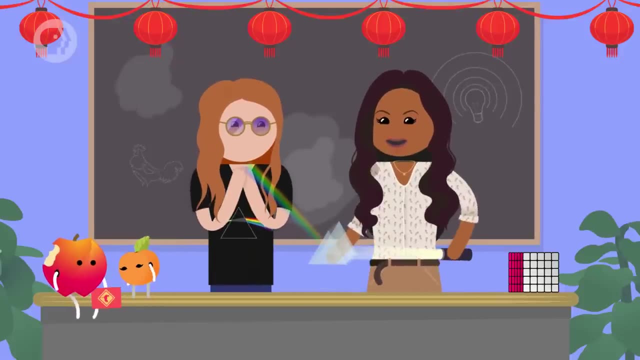 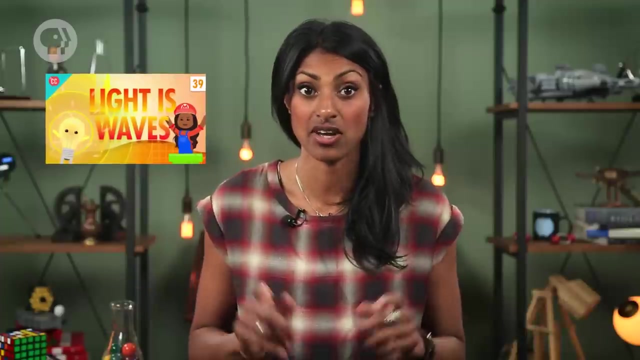 Light is everywhere, but it's not as predictable as you might think. It's a wave that travels in straight lines, yet it also reflects off surfaces, refracts through various materials and generally changes direction all the time. We've learned how to bend light to our will with lenses and mirrors, but it's time to take a step back and ask what we can learn from light. 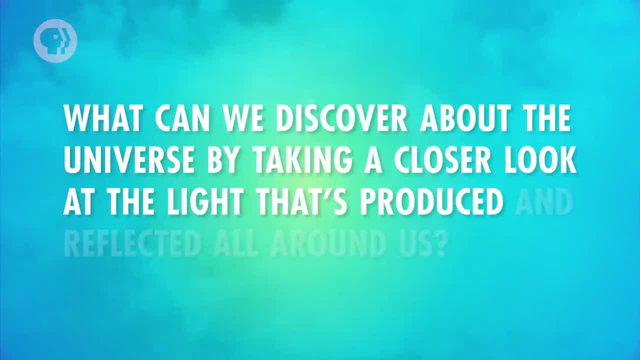 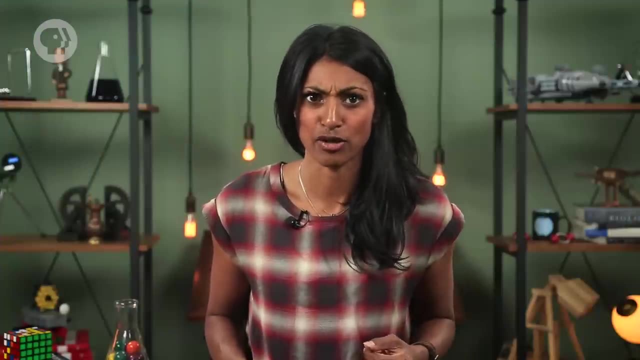 What can we discover about the universe by taking a closer look at the light that's produced and reflected all around us? It's time to use our understanding of the wave nature of light to explain what stars are made of, why you see rainbows in an oil stain in the parking lot. 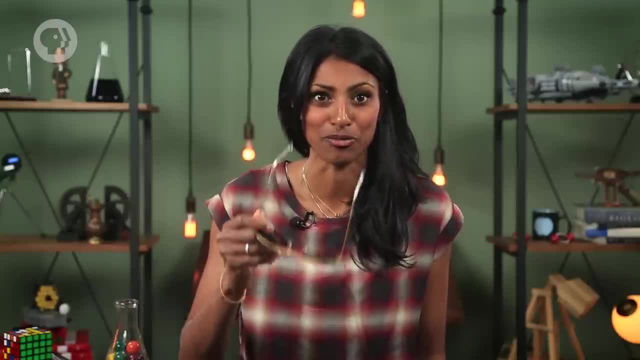 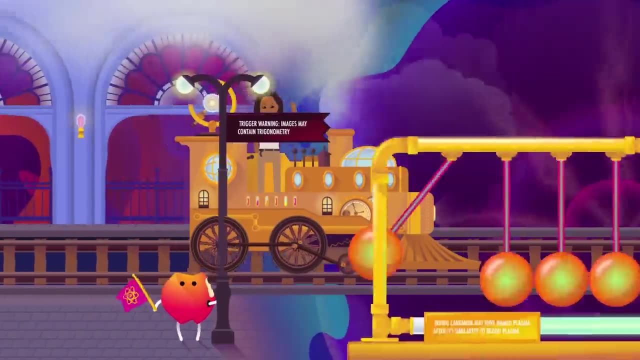 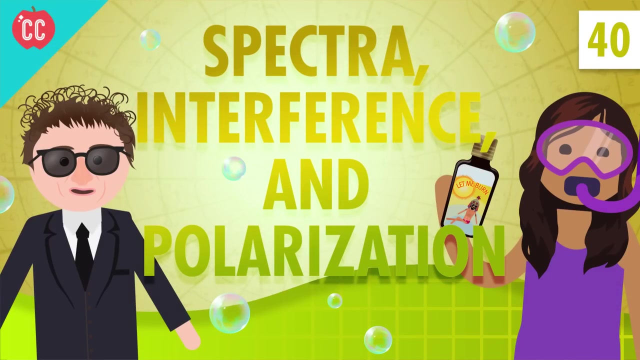 and how some fancy sunglasses can make a bright day a lot more bearable. In order to unlock the secrets that light can reveal to us, we need to look again at diffraction. We need to look again at diffraction. We need to look again at diffraction. 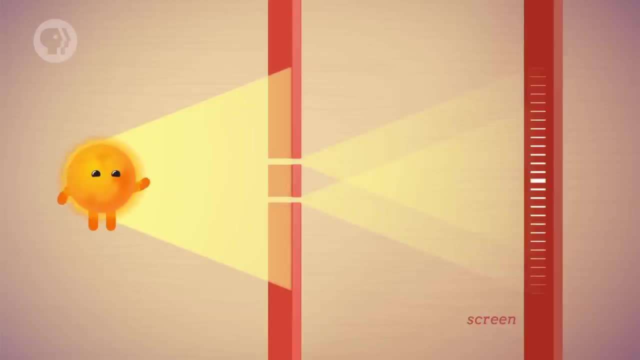 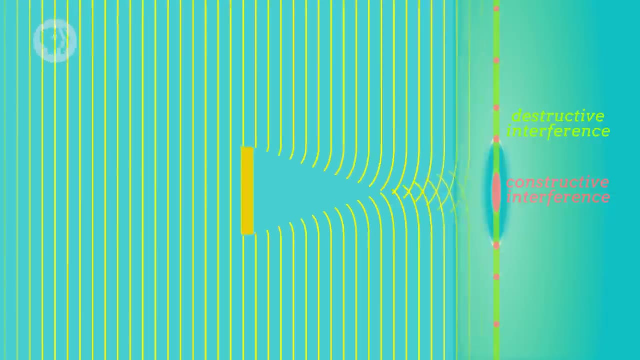 Remember. That's what causes the pattern of lines that appear when you shine a light through a pair of thin slits. The bright lines are the result of constructive interference when light waves build on one another, while the dark spaces in between are the result of destructive interference. 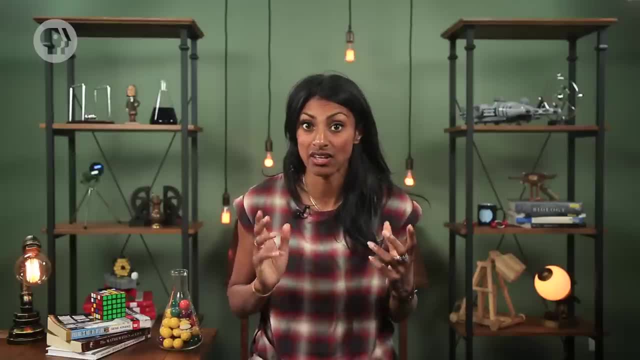 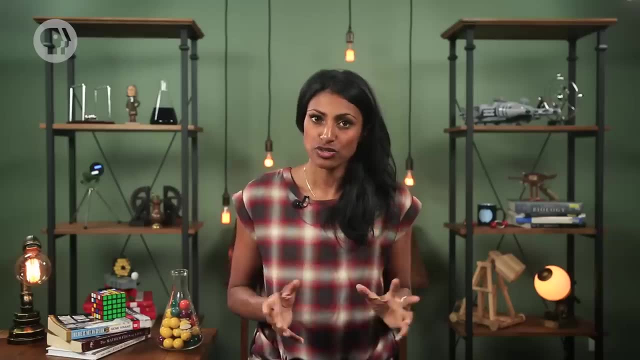 Exactly how this diffraction pattern looks depends on the spacing of the slits and the light's wavelength. So if you know the distance between the slits, then you can measure the diffraction lines to get some information about the light source. Now you can also shine light through many equally spaced slits. 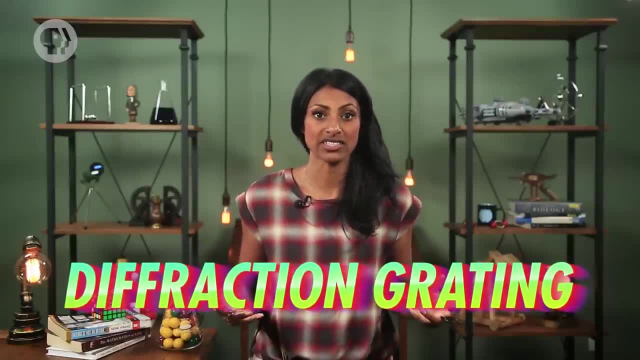 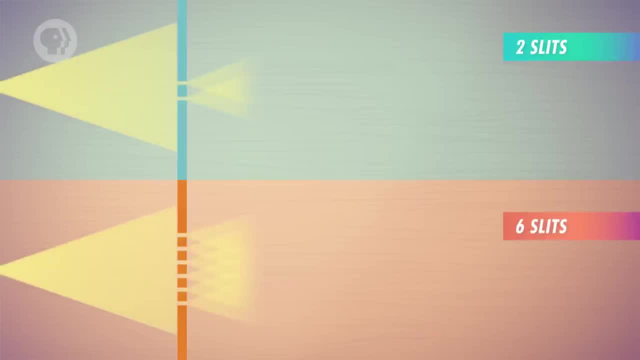 This is called a diffraction grating, And when you shine a light through one of these gratings, the diffraction lines are much more intense and easier to measure. Plus, when there are more slits, there's also more opportunity for destructive interference. 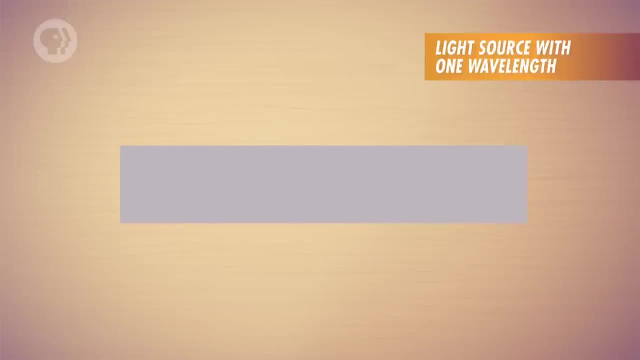 so the dark spots between bright lines are larger as well. Now, if the light source has light of only one wavelength, which is one distinct color, then all the lines would be the same color and would be evenly spaced. But if you have a light source with two wavelengths, 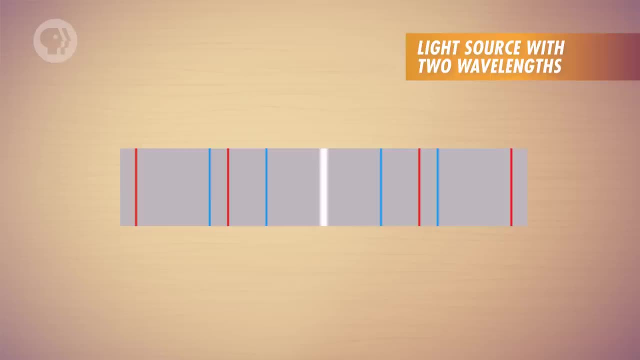 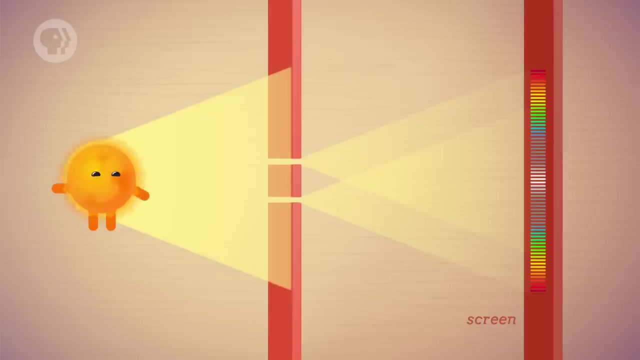 then you'll get multiple sets of bright lines whose color and locations will depend on the wavelength. And if your light source is white light containing all visible wavelengths, then you'll see a little rainbow in the place of every bright line, because the grating is separating out each wavelength. 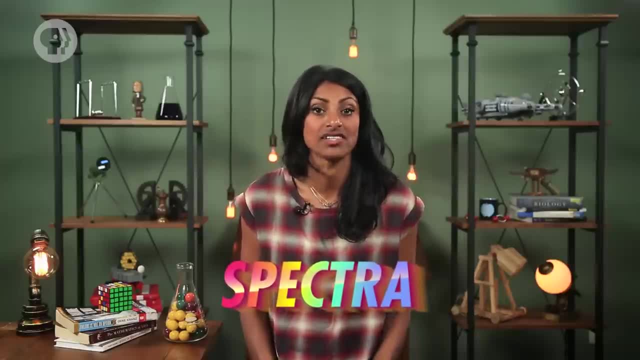 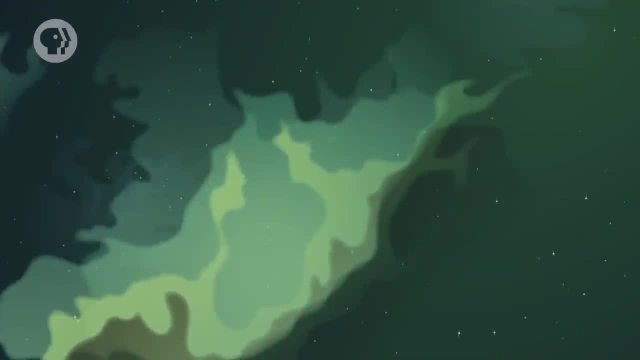 These patterns are known as spectra, and you can study them to learn about the source of the light. To do that, you need a spectrometer, a tool that uses diffraction grating or a prism to separate the wavelengths. Let's say that you heat up a cloud of hydrogen until it emits light, and then you point your spectrometer at the cloud. 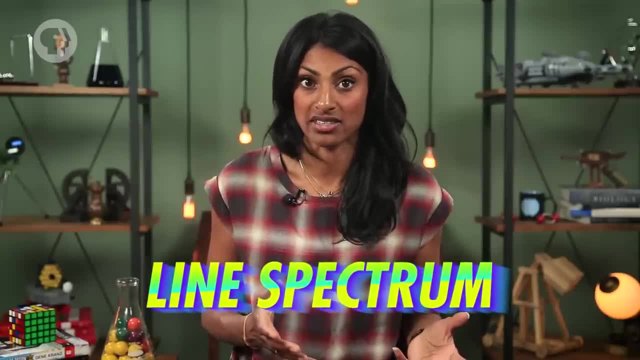 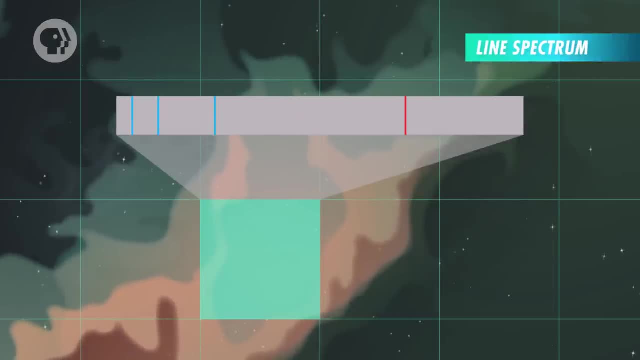 The gas will emit a line spectrum, a distinct pattern of lines at certain wavelengths that correspond to the elemental composition of the cloud, In this case hydrogen. The spectrum would look like this And you'd always see this line spectrum from a heated hydrogen cloud or a compound that contains hydrogen. 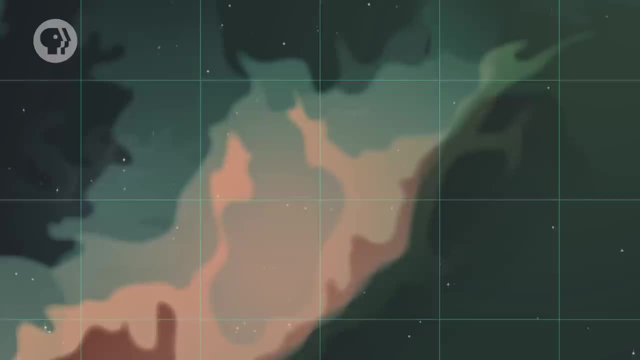 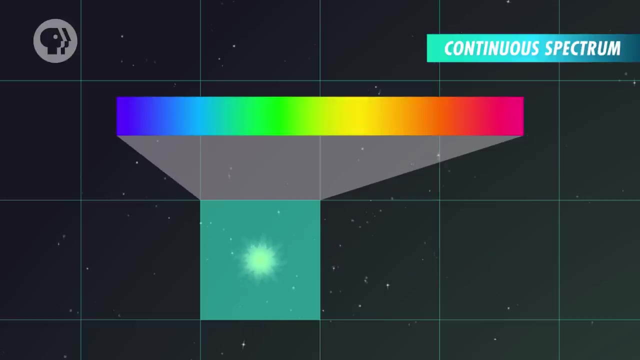 Line spectra work for heated gases under the right low-pressure conditions, But when solid materials or high-pressure gaseous objects like the sun get heated up, they emit a continuous spectrum of light that covers a very wide range of wavelengths, And in that case you can still get information about the light source. 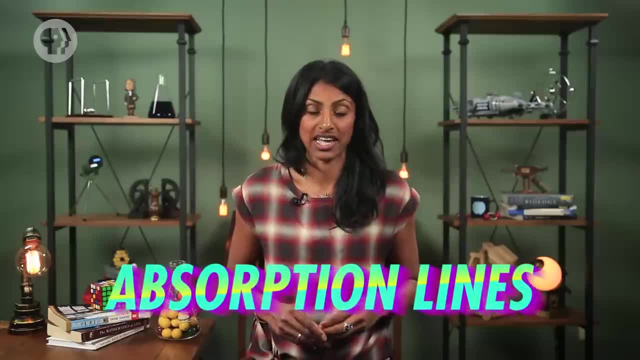 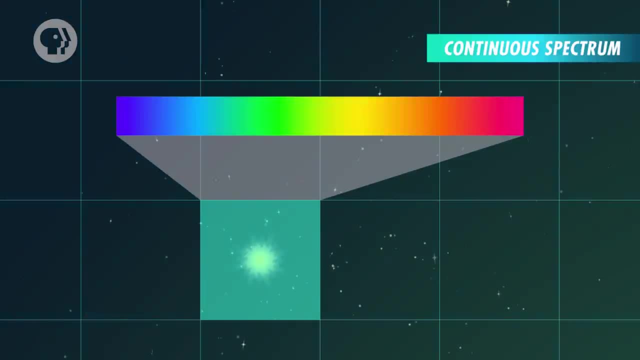 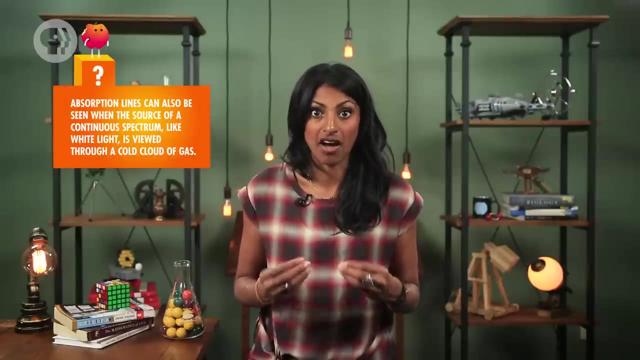 because the continuous spectrum from a heated object also contains absorption lines, characteristic wavelengths of light that have been absorbed by the same elements that emitted them. The sun emits a continuous spectrum, but some elements in its atmosphere absorb some of the light. Hydrogen atoms, for example, absorb light emitted by other masses of heated hydrogen. 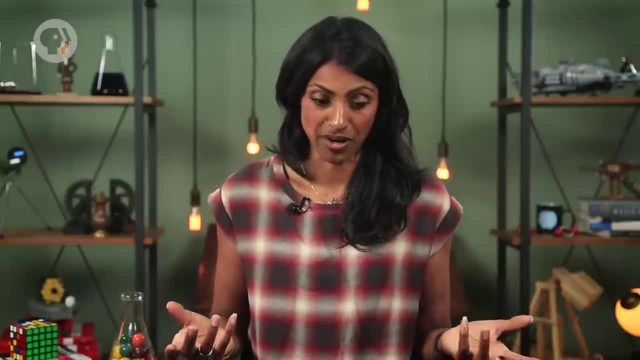 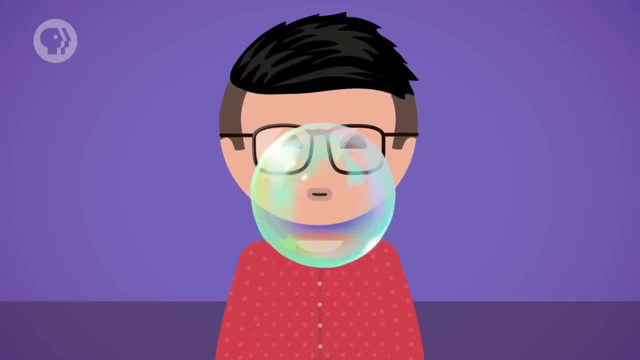 But you don't always need special equipment to see and study continuous spectra. Have you ever blown a soapy bubble and noticed the bright rainbow colors on its surface? That coloring is also due to interference and the separation of wavelengths, an effect known as thin-film interference. 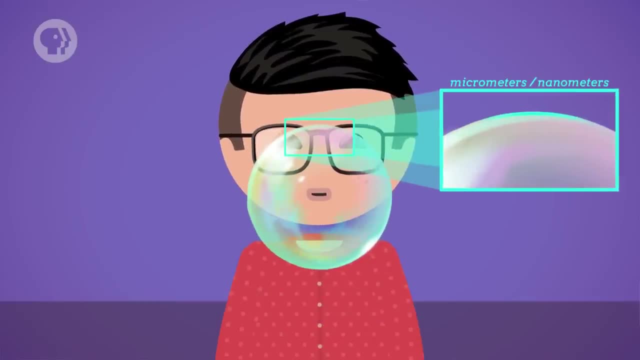 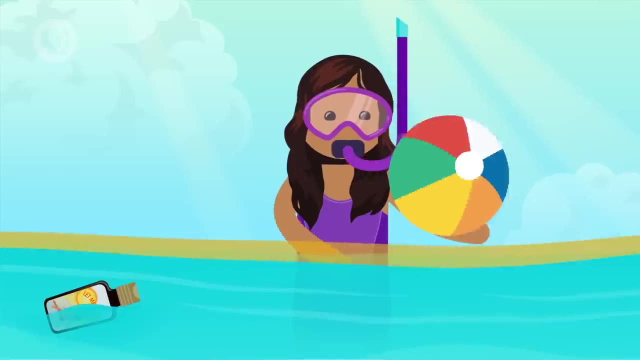 Thin films are layers of materials whose thickness can be measured in micrometers or even nanometers of the order of a wavelength of visible light. For example, a layer of oil on top of water could be a thin film. Imagine such an arrangement of oil and water with a ray of white light coming down from above. 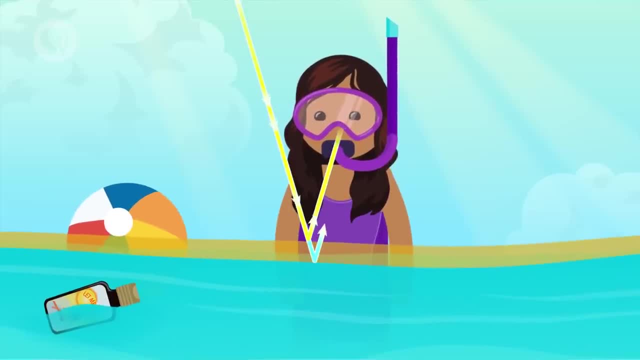 We know that some of the light will reflect off the top of the oil and some will pass through. Of the light that goes through the oil, some of it will reflect off the surface of the water. Now, the light that's reflected off the oil will interfere with the light that's reflected off the water. 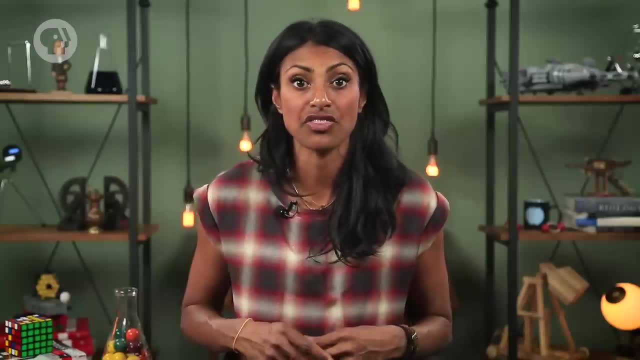 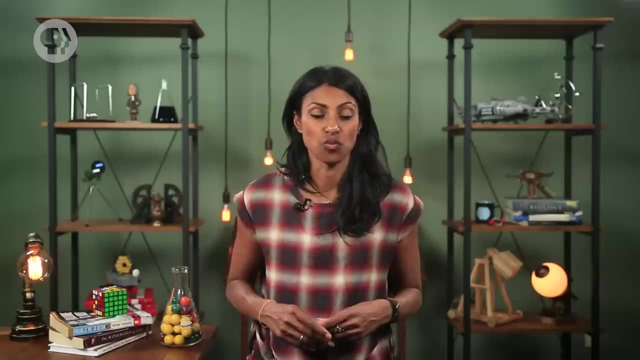 And whether that interference is constructive or destructive depends on the thickness of the oil and the light's angle of incidence. So ultimately you end up with both kinds of interference. Each kind occurs only for certain wavelengths of light, depending on the angle at which it's viewed. 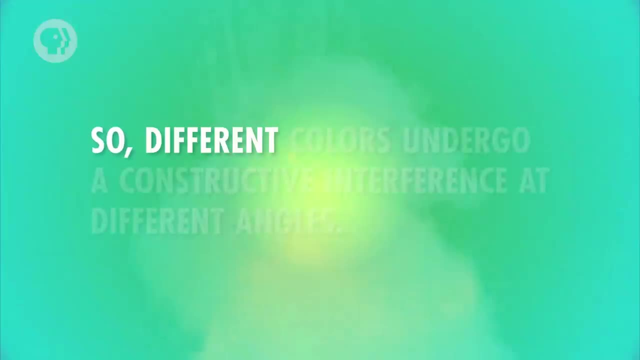 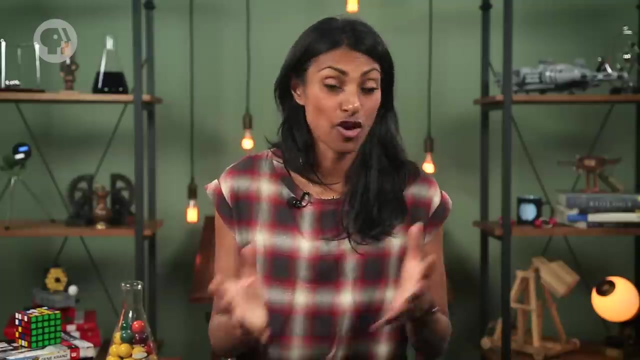 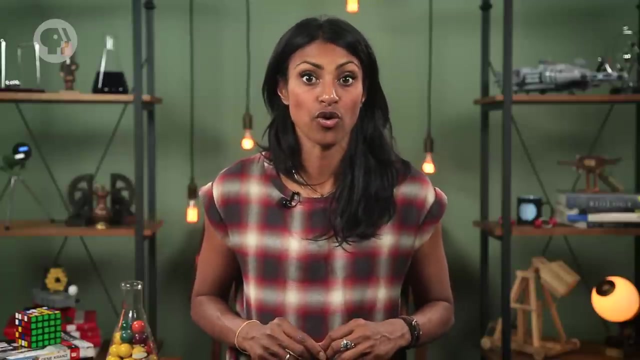 Because as the viewing angle changes, so does the path length, So different colors undergo a constructive interference at different angles. The result is an alternating pattern of colorful reflected light and no reflection at all. Constructive interference creates a visible colored reflection, while destructive allows light to go through the oil to the water. 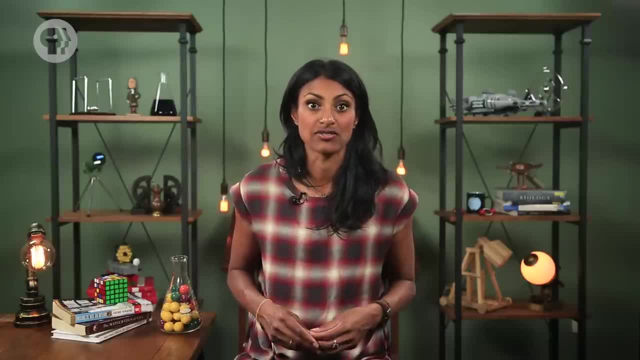 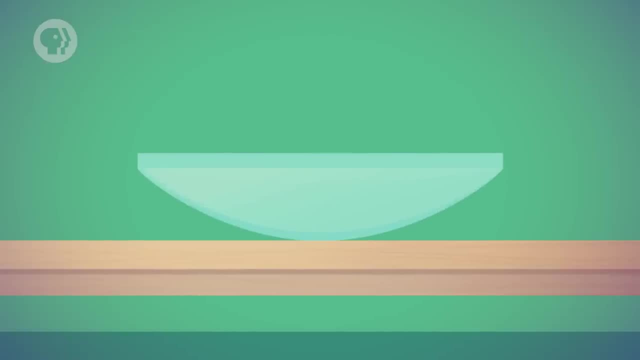 This phenomenon happens not just with layers of liquid, but also with layers of some transparent solids, namely glass. You can create a similar effect if you have a lens with one flat side and one curved side and you put the curved side on a flat plate of glass. 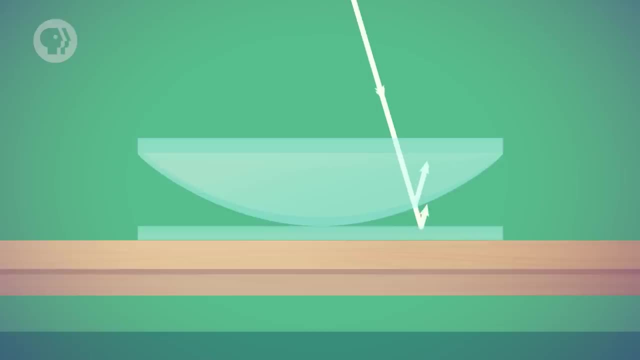 As light shines from above and enters the flat side of the lens, some rays reflect off the bottom of the curved lens, while others pass through into the thin gap of air that sits between the lens and the plate. That light then reflects off the bottom plate and returns back through the lens. 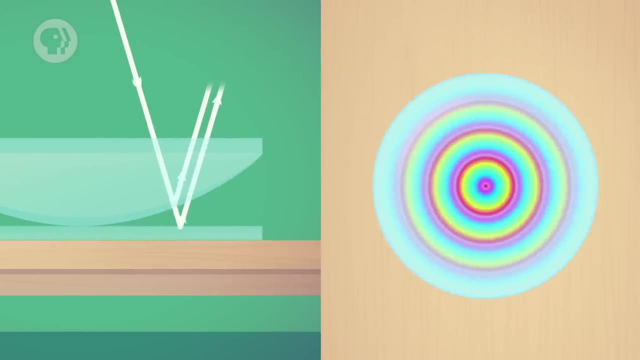 The resulting interference creates a circular rainbow pattern that extends out from the point of contact between the lens and the plate. These circles are known as Newton's Rays And if the light source is monochromatic, the rings simply alternate light and dark, displaying alternating constructive and destructive interference. 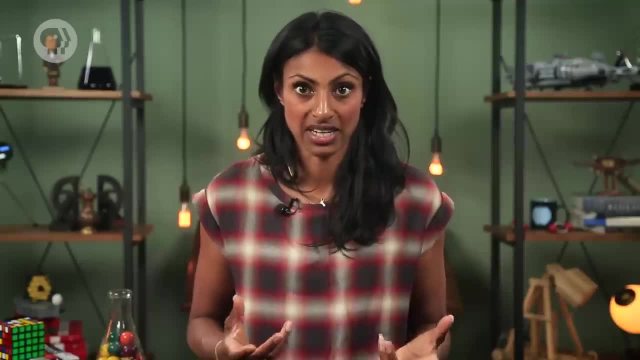 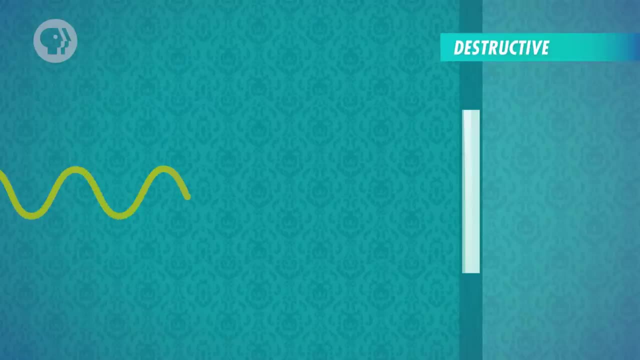 Now, if you look at the very center of Newton's rings, where the glass plate is in contact with the lens, you'll notice a dark spot. That's where the reflected wave of light is not constructively interfering with itself. Instead, at this point of contact, the reflected ray undergoes a phase shift of 180 degrees, essentially skipping forward half a cycle. 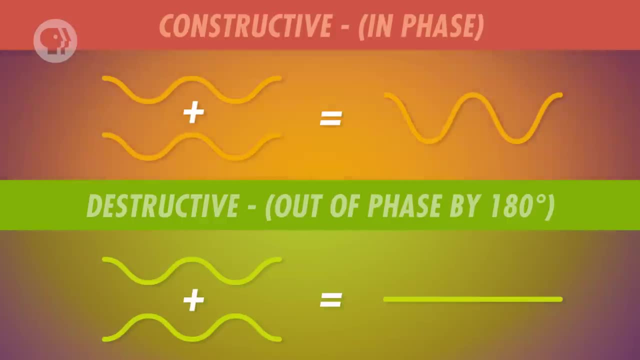 Remember, when a wave is in phase with another wave, their crescent troughs are amplified, meaning the light is brighter than the light source, And when a wave is out of phase by 180 degrees, it's destructive, with the crescent troughs cancelling each other out. 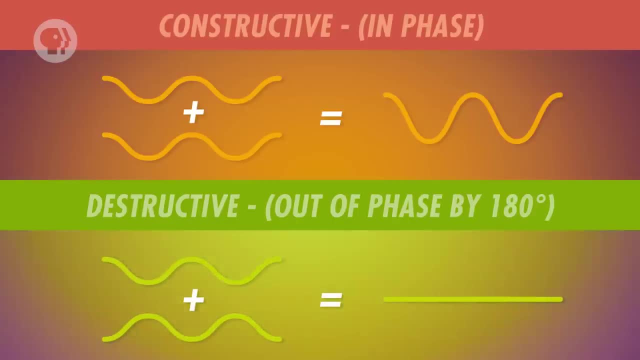 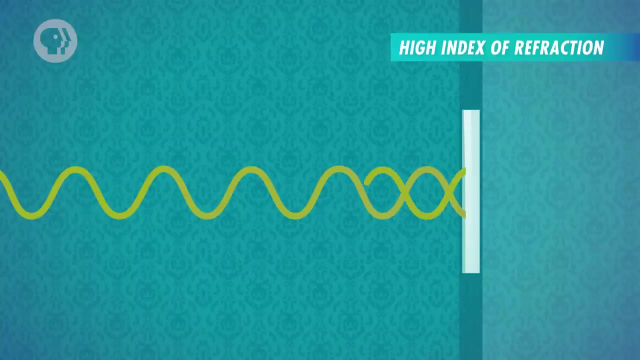 The resulting destructive interference is seen in the dark spot at the center of the lens. When light reflects off a surface that has a higher index of refraction than the medium it travels through, such as light traveling through air and reflecting off glass, the ray undergoes a destructive 180-degree phase shift. 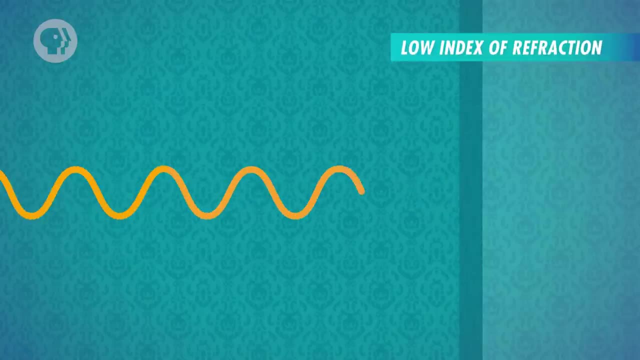 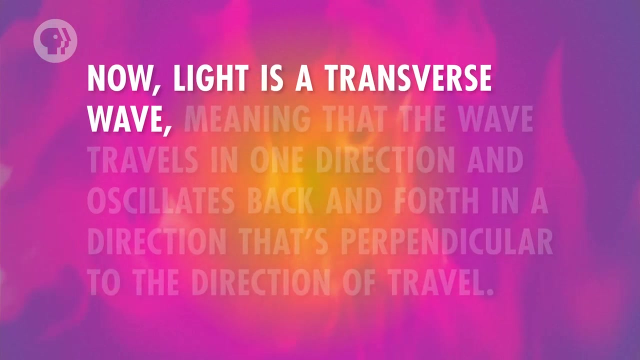 But if the light reflects off a surface that has a lower index of refraction than the medium it's passing through, there is no phase shift and the wave then constructively interferes with itself. Now, light is a transverse wave, meaning that the wave travels in one direction and oscillates back and forth in a direction that's perpendicular to the direction of travel. 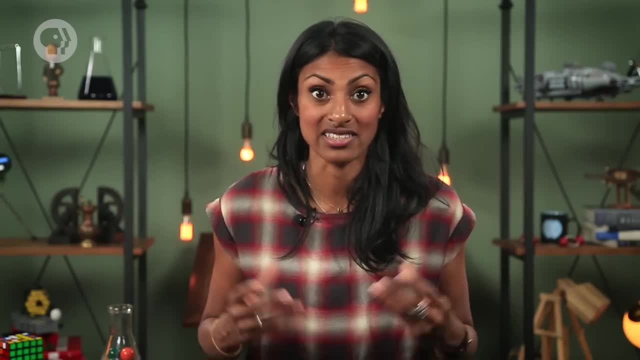 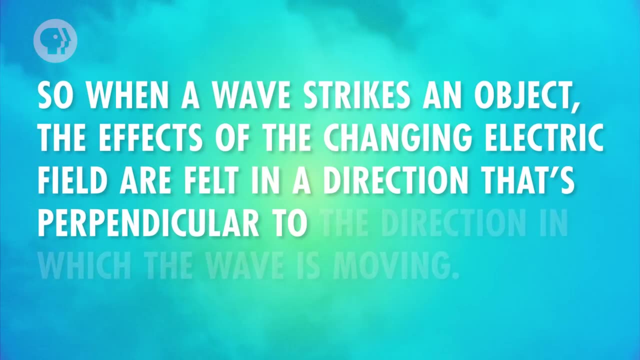 And, like all electromagnetic waves, what's oscillating in a light wave is its electric field. So when a wave strikes an object, the effects of the changing electric field are felt in a direction that's perpendicular to the direction in which the wave is moving. 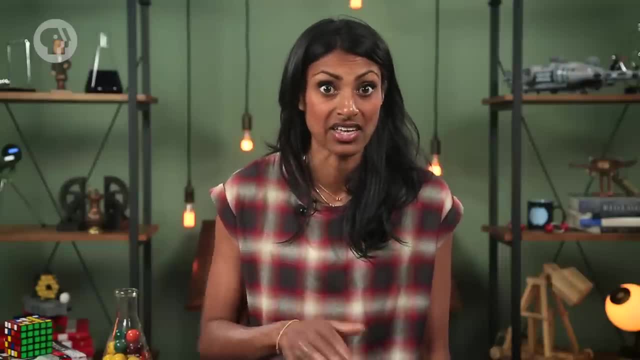 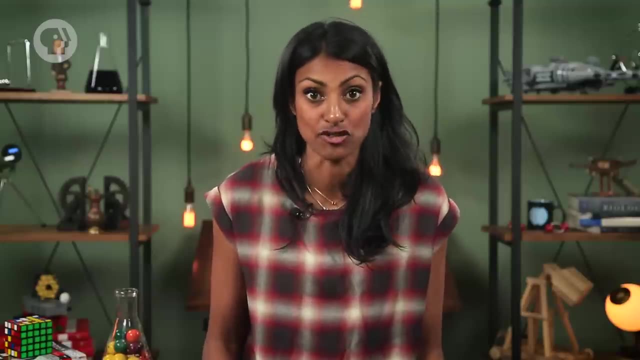 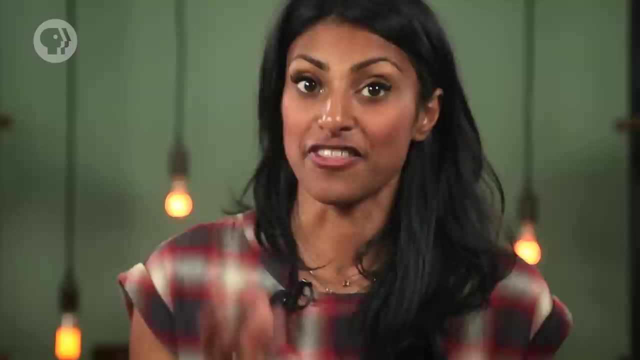 But a light wave's electric field can not only move vertically, that is, up and down. It can also oscillate horizontally Or side to side, since that movement is still perpendicular to the direction of travel. This oscillation is important because you can limit what light passes through a filter depending on what direction its electric field is oscillating in.